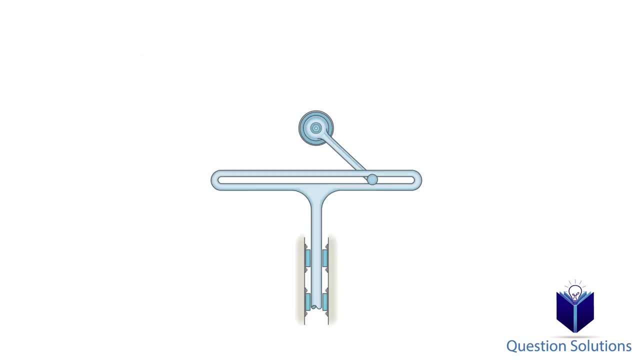 and rotation about a fixed axis. Now let's get started with a few examples, and by the end you should be able to solve the problems you will face in this chapter. Let's take a look at this question and the diagram to understand what's happening here. 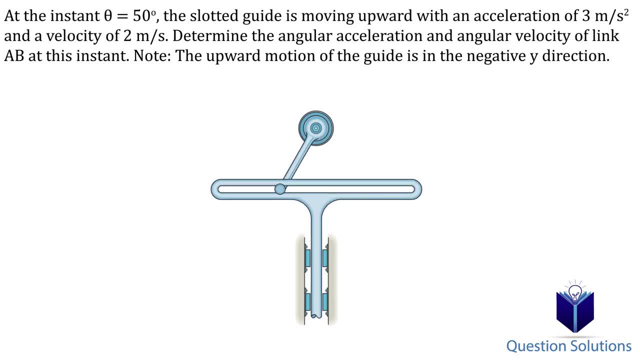 When the link AB is moving along the slot, the slotted guide moves upwards. When the link moved 50 degrees, the slotted guide has a velocity of two meters per second, with an acceleration of three meters per second squared. So we see that the slotted guide moves up and down while the 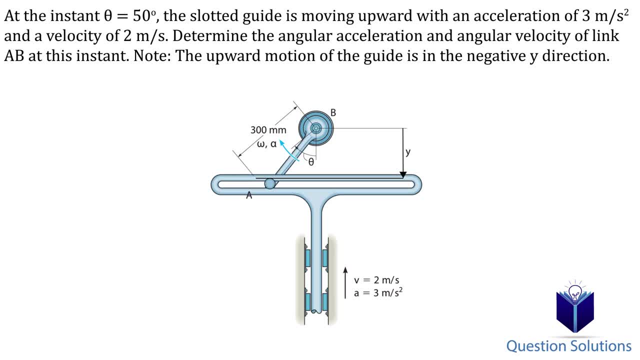 link is moving in a circular pattern, So what we need to do is figure out a way to relate the rotational movement of the slotted guide to the slotted guide. Let's take a look at this question and the diagram to understand what's happening here. When the link AB is moving along the slot, 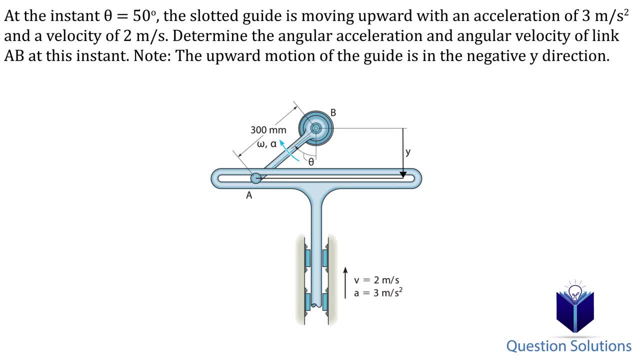 the slotted guide moves upwards When the link AB is moving in a circular pattern. So we can use the length y already marked on the diagram to figure this out. We see that as the angle changes, length y also changes, so they are related. This y-length or displacement tells us where the 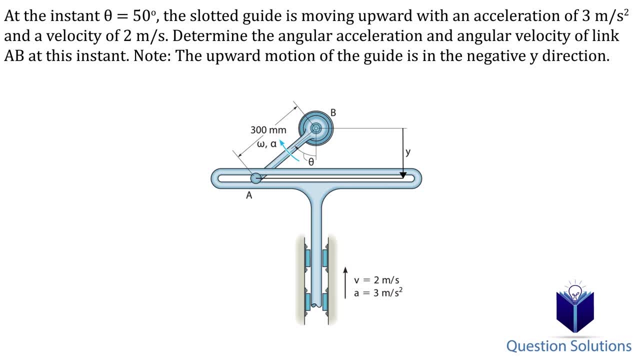 slotted guide is with respect to the angle of the link. So how can we express the length of y with respect to the angle? We can use trigonometry. We can form a right-angle triangle like this and one side of it will be the slotted guide and the slotted guide will be the slotted angle. So we 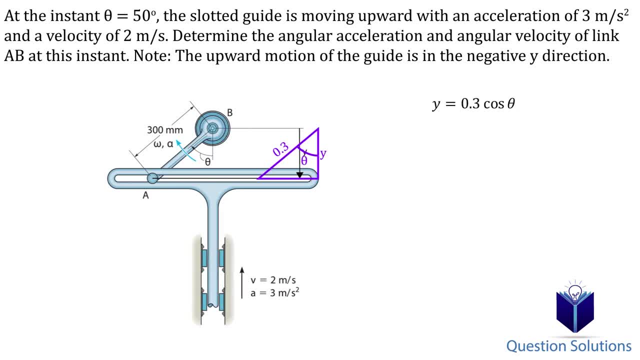 can write. y is equal to 0.3 cosine theta. Note that we converted 300 millimeters to meters. Now it's just a matter of taking derivatives with respect to time. If you don't remember or need a refresh on how to do this, please check the description. We will take the first derivative. 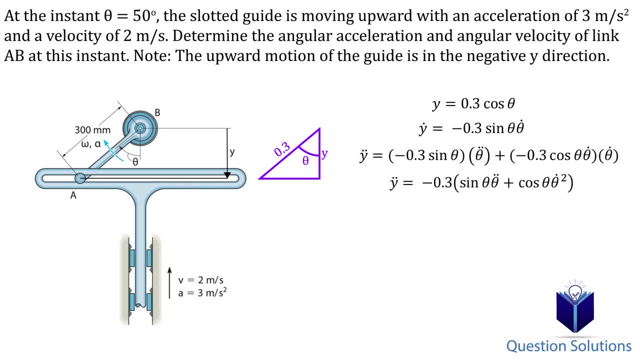 now the second derivative. Let's simplify it. It's important to realize that this y-value is actually a displacement. It measures where the slotted guide is. So we can use trigonometry to find out where the slotted guide is. So we can use trigonometry to find out where the slotted 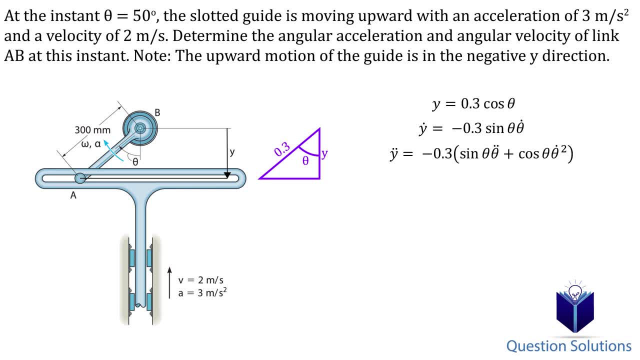 piece is with respect to the link. That means one derivative of it gives us velocity and the second derivative gives us acceleration. So y with one dot on top is actually velocity and y with two dots on top is acceleration. Again, this velocity and acceleration is of the slotted guide. 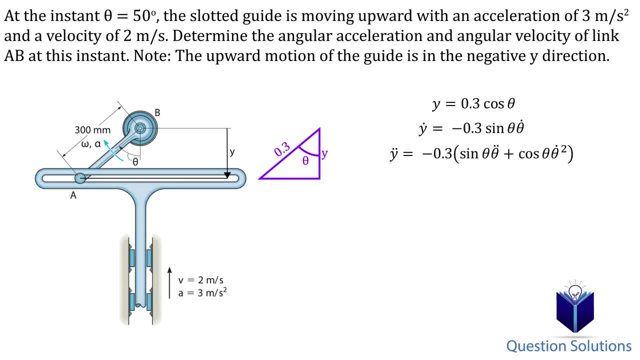 not the link. Also, remember that theta with one dot on top is angular velocity and theta with two dots on top is angular acceleration. Now we're ready to plug values in. We will start off with the velocity equation. So the velocity is negative two meters per second. 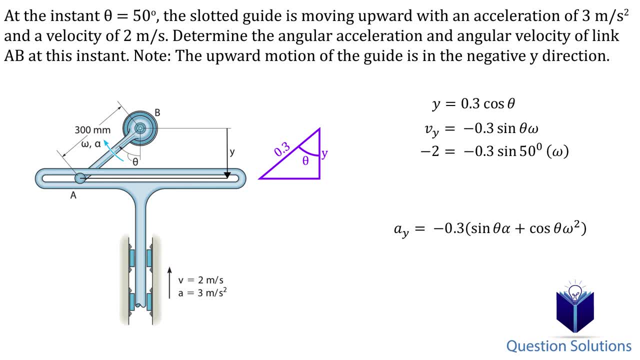 and the angle is 50 degrees. The velocity is negative because we're told the upward motion of the guide is in the negative y direction. Let's solve for the angular velocity. Next angular acceleration. The acceleration is negative, three meters per second and the angle is still the. 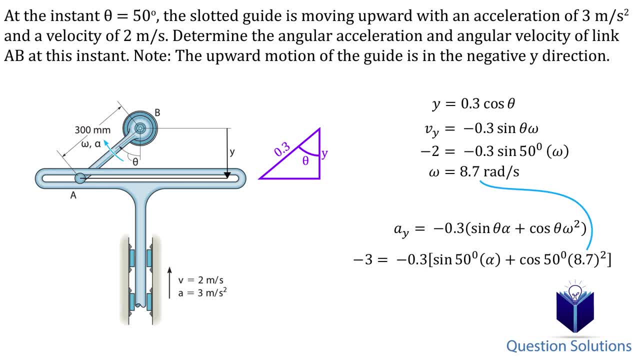 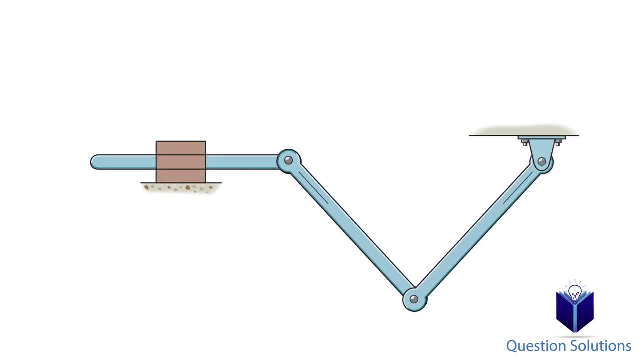 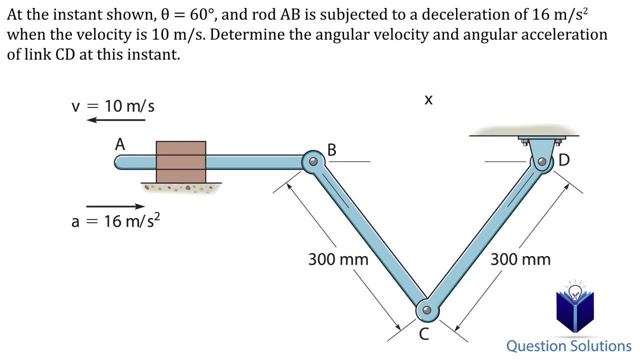 same. Don't forget to plug in the angular velocity we just found. Let's solve for the angular velocity. Those are our answers. Let's take a look at this example where we need to figure out the angular velocity and angular acceleration of link CD. We see that link AB moves back and forth when 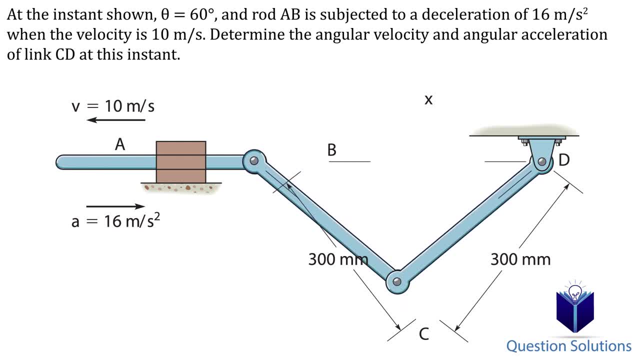 the other two links move in their own respective path. So the goal is to relate the movement of link AB to that of link CD. From the fixed point at D we can see that the horizontal distance to point B changes depending on the position of the links. So we can use this equation to calculate the 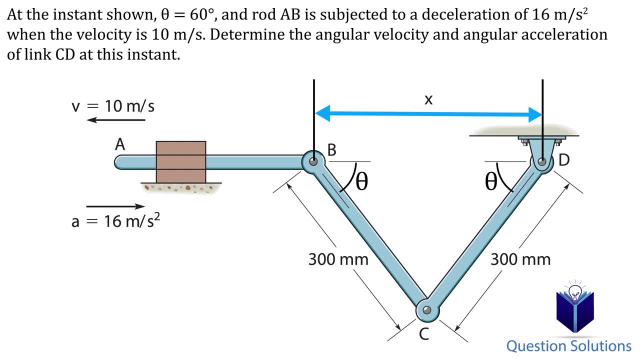 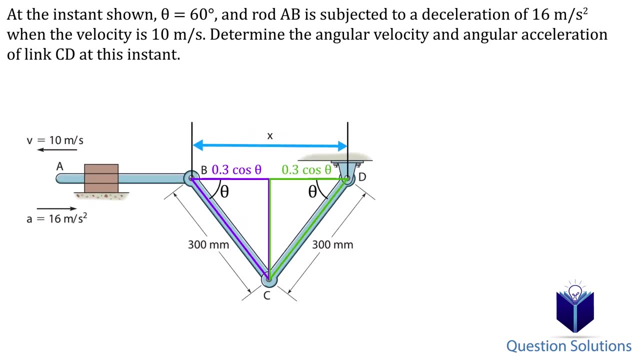 angular velocity. We can use that distance and relate its length with the angle. the link CD and CB makes. Let's use trigonometry to figure it out. Notice how we can draw two right angle triangles like this. So the base of each triangle would be 0.3 cosine theta. The total distance is then two. 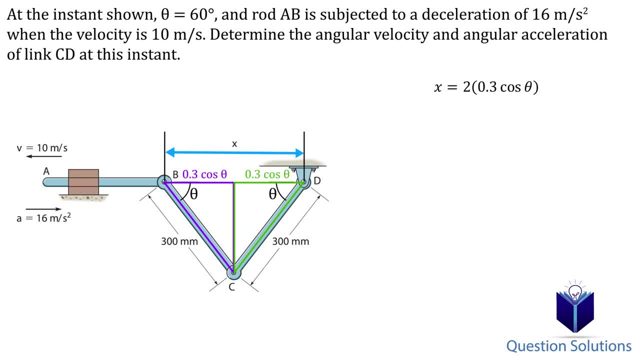 times that, since we have two bases. So now we can take the derivative. Now for the second derivative. Let's simplify while at the same time switching out the theta dots with the angular velocity. Now we can plug our values in starting with velocity We're going to assume left to be. 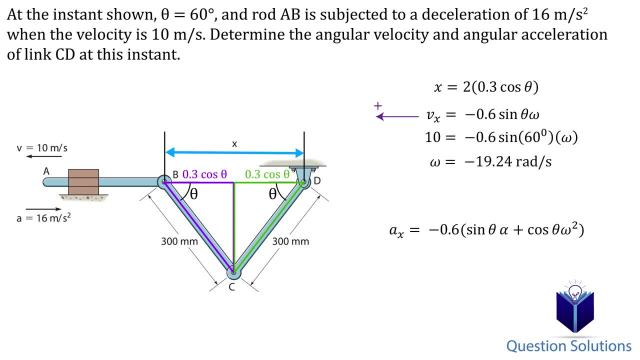 positive, Let's solve for the angular velocity. Next acceleration: Let's plug in the values we know, along with the angular velocity we just found. Remember we picked left to be positive and since it's a deceleration for rod AB, it's negative. Let's solve for the angular acceleration. 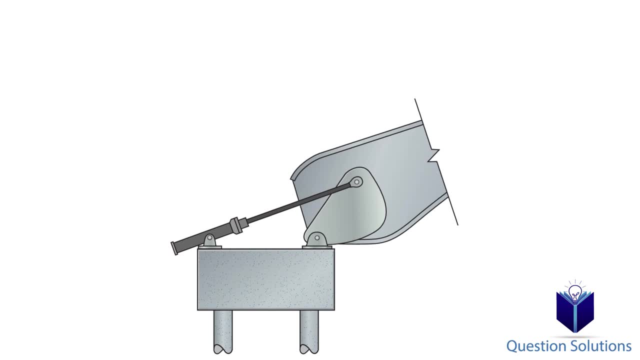 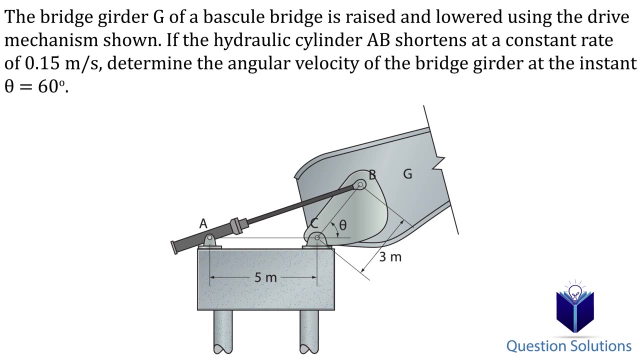 Those are our answers. Let's take a look at this question where we need to figure out the angular velocity of the bridge girder. So the first step is to relate the displacement of the hydraulic cylinder AB to the angle, So we can measure the distance from point A to B with respect to the angle.